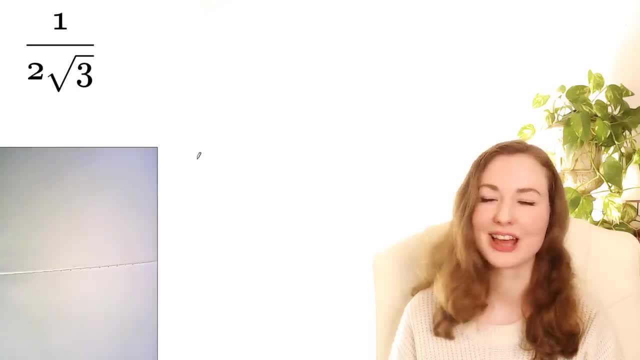 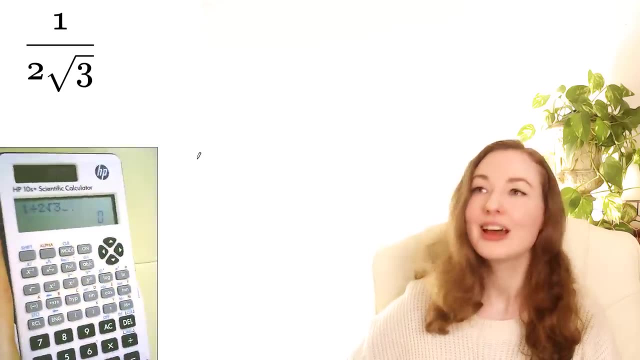 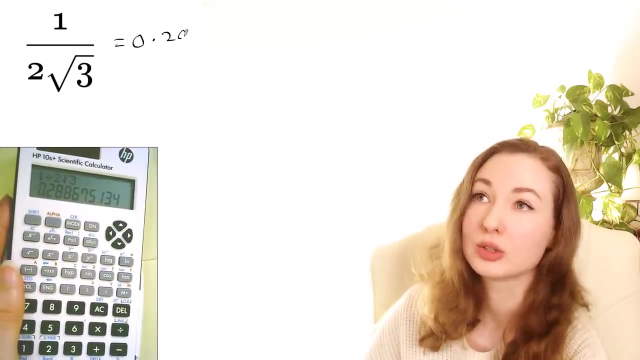 Let's suppose you're in an exam and you need to calculate 1 over 2 root 3.. So you're used to putting this into your trusty calculator as 1 divided by 2 root 3, like that, Hit equals and you would get the correct answer of 0.29.. But let's suppose on this particular day your calculator has 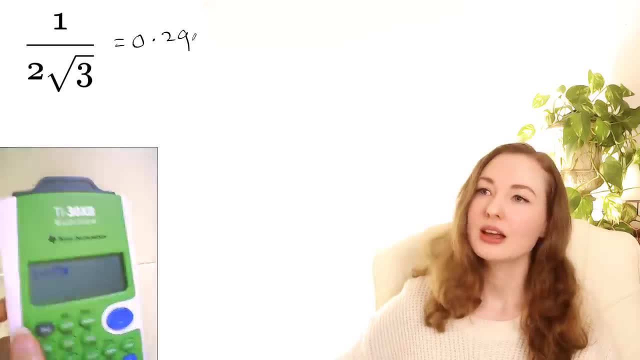 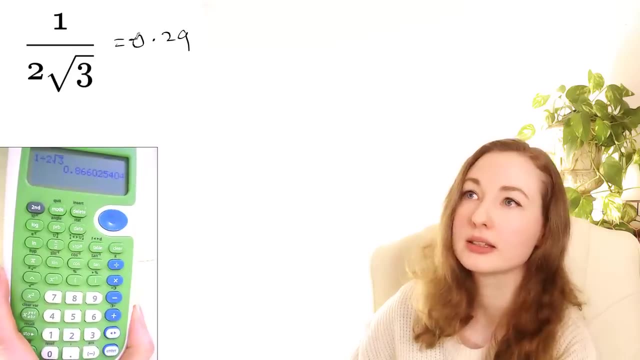 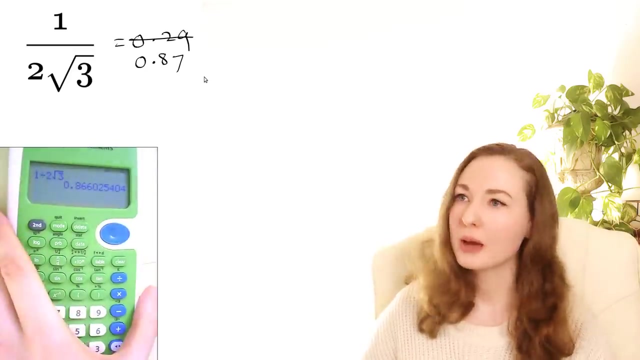 run out of batteries and you borrow a friend's calculator. So you type it in as you normally would: 1 divided by 2 root 3, and hit enter, and you get 0.87, which is incorrect if that's what you're trying to calculate. So what's happening here? Well, this calculator is interpreting this. 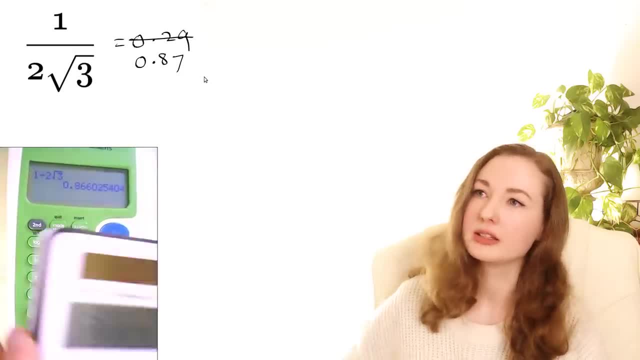 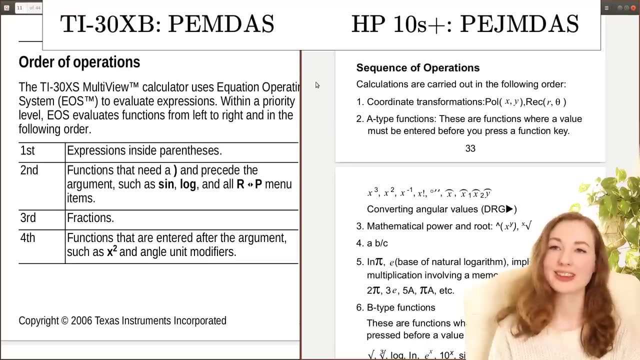 as half of root 3, whereas the HP interprets it as it's written there. So to find out why this happens, let's have a look at the manuals. Now, when we write something like 2 root 3 without any kind of multiplication symbol in between the 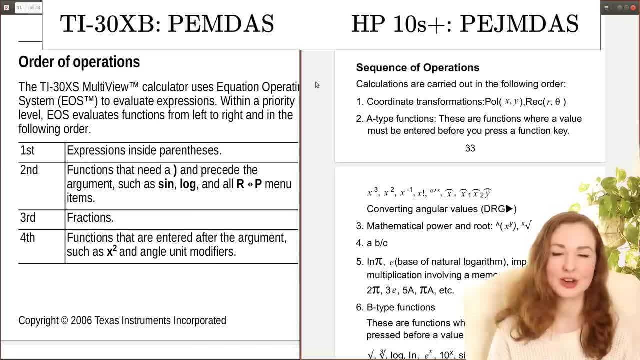 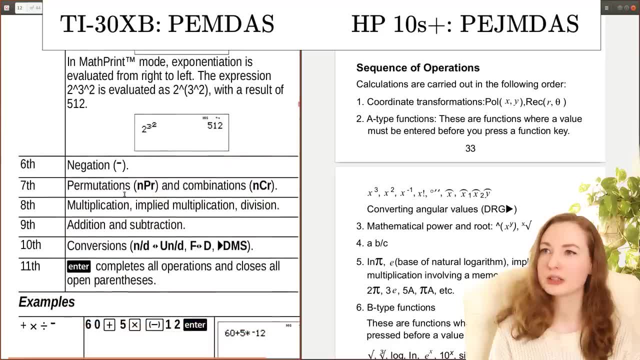 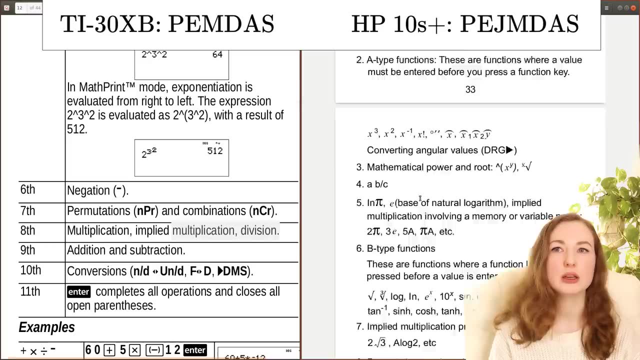 2 and the root 3. that's called multiplication by juxtaposition or implied multiplication. So on the TI's manual, under order of operations, it has the implied multiplication at the same level as division, whereas for the HP it has a couple of extra levels, has implied multiplication. 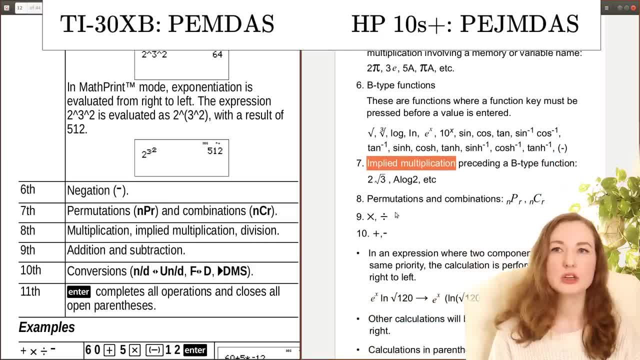 there And also here, Whereas division is all the way down here. So this method, where implied multiplication has the same priority as division, I'm going to be calling that PEMDAS. This one where there's this extra level, I'm going to be calling that PEDIMDAS. 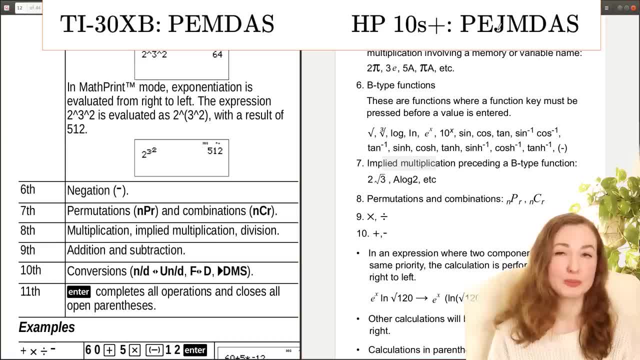 So, parentheses, exponents, multiplication by juxtaposition, and then multiplication and division- so explicit multiplication with the time and division- so explicit multiplication with the time. So this is going to be called PEDIMDSAS. So this is going to be called PEDIMDSAS. 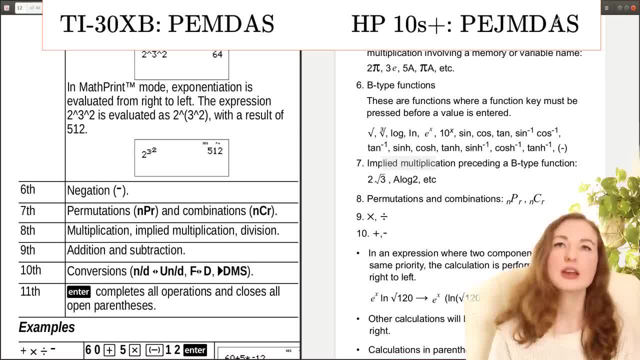 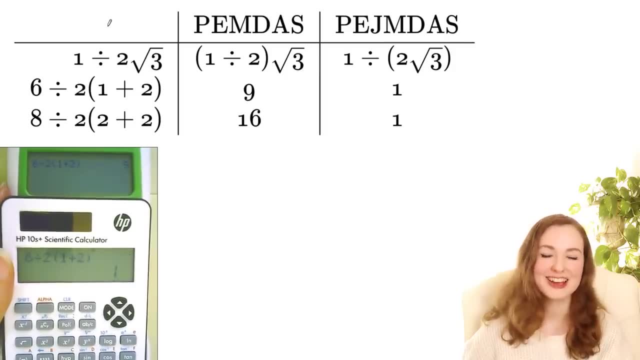 So this is going to be called PEDIMDSAS symbol. that still has the same level as division, and then there's addition and subtraction. So those are the two main methods that calculators use, either PEMDAS or PEJMDAS. So this disagreement between PEMDAS and PEJMDAS is: 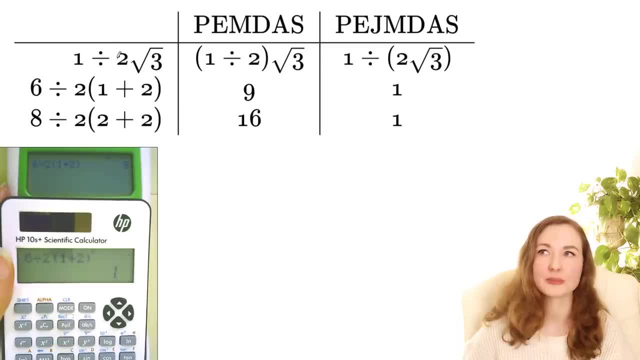 what causes the two calculators to interpret this differently. It's also what causes them to interpret the one of the famous Facebook questions differently. These things keep popping up. I think the current iteration is this: 8 divided by 2 times 2 plus 2.. But when I made my first video on PEMDAS about this, 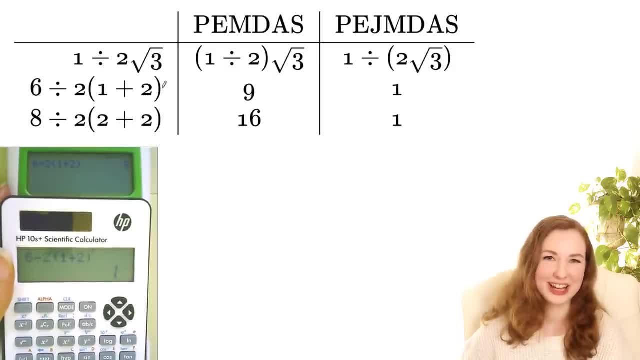 question. a lot of people were just saying: you know who cares, it's just a silly Facebook question. But I'm hoping that by showing the different ways that the calculators interpret this, it demonstrates that this is actually kind of a problem, because students could be losing marks, And not just that. 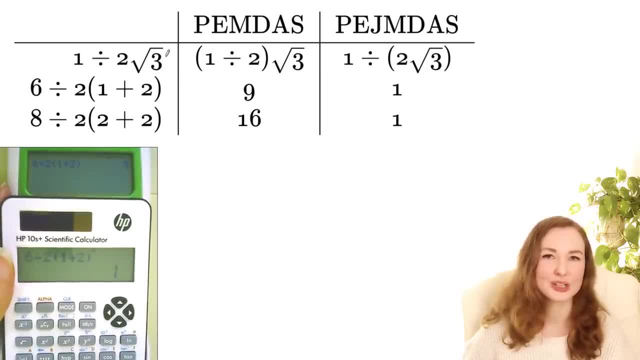 but I don't know if you've ever been in a situation where you're trying to work through a textbook and your answer to a question doesn't match what's in the back of the book and you keep checking and rechecking it and rereading the 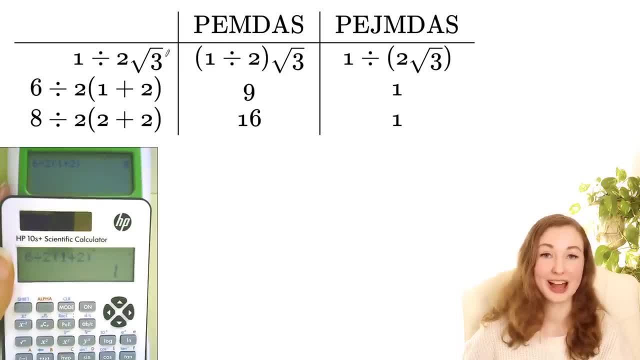 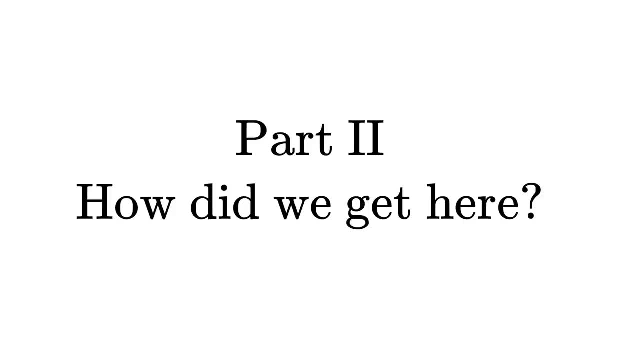 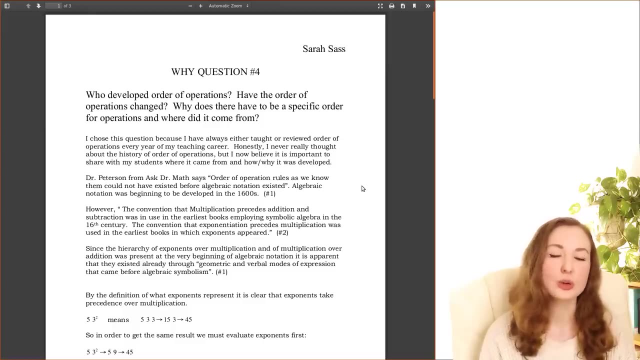 chapter, and that can just take hours out of your life. So I think this is actually kind of a problem. So let's have a little look into the history of PEMDAS. Now, I wasn't able to find out who invented the answer to the question. 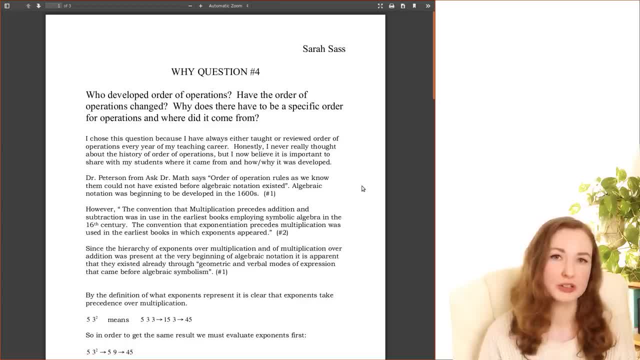 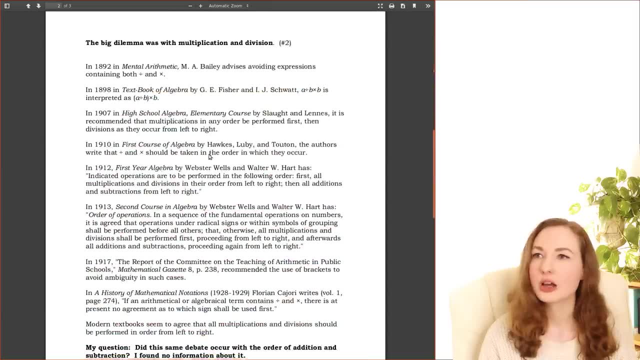 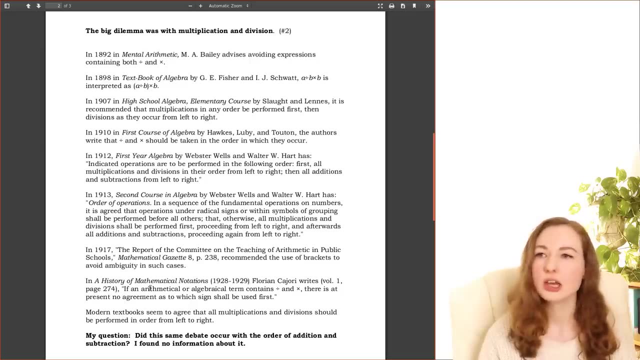 acronym itself, but the idea that multiplications and divisions have the same precedence. Let's have a look at that. So there's this article by Sarah Sass which goes over quite thoroughly the history of this. Now, right into the 1920s, there wasn't any sort of agreement about the order that they should be done. 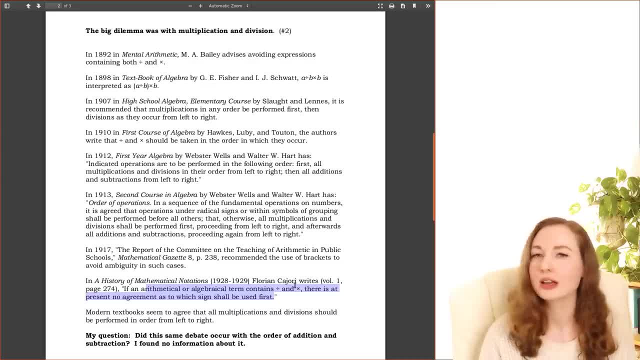 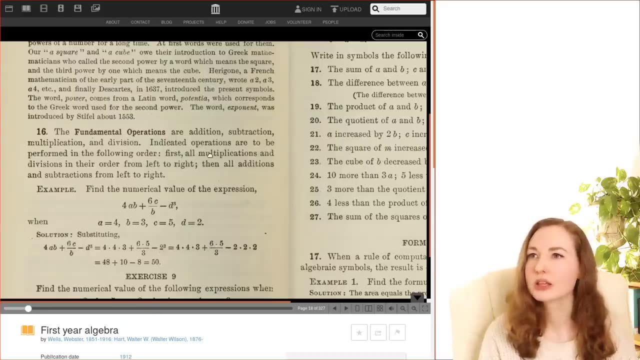 in. Some authors were saying multiplication should be done first and others were saying that they should be done in the order they occur. So there's these three books that are putting forth that idea, this PEMDAS idea. Now let's have a look at them. So first year, algebra, that's saying all multiplications. 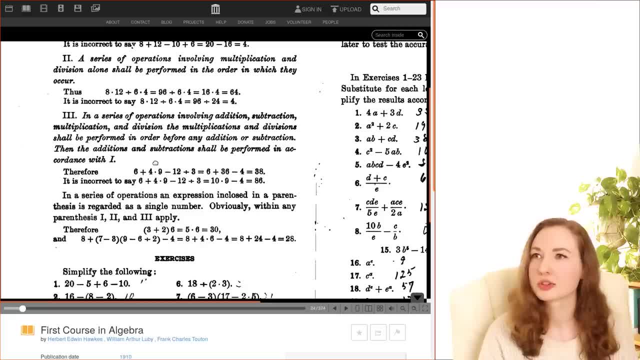 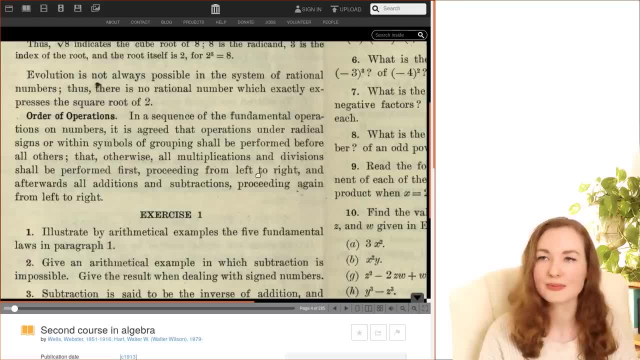 and divisions, in their order from left to right. Then there's first course in algebra, which says something similar, and second course in algebra- similar thing again. Now, what's really interesting, though, is that, if you actually read through these books, all three of them break that rule when it comes to 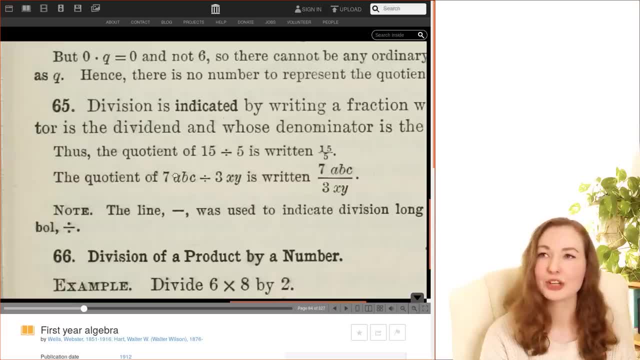 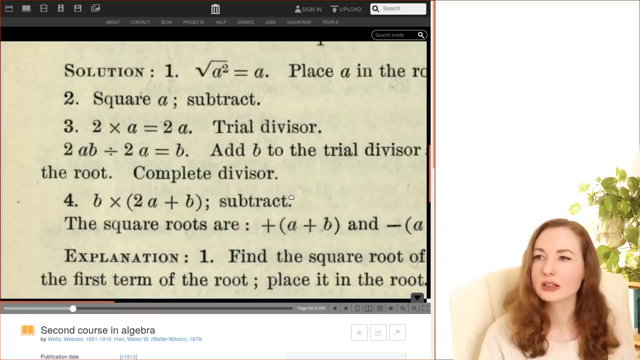 juxtaposition. For example, in first year algebra you see expressions like this being taken to mean this, which is actually following PEMDAS. In first course in algebra you see a similar kind of thing and in second course in algebra we've got this: 2ab divided by 2a, making b. Now if you followed the rule that they 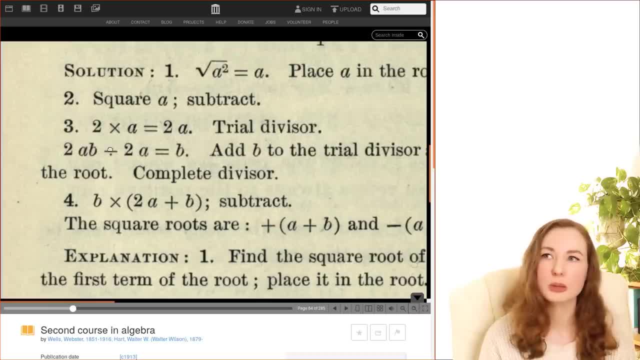 had stated to the letter, you would interpret this as 2ab divided by 2b Divided by 2, so you work out that that's ab and then you multiply by a, so you get a squared b and not b as they've written here. So why haven't they stated? 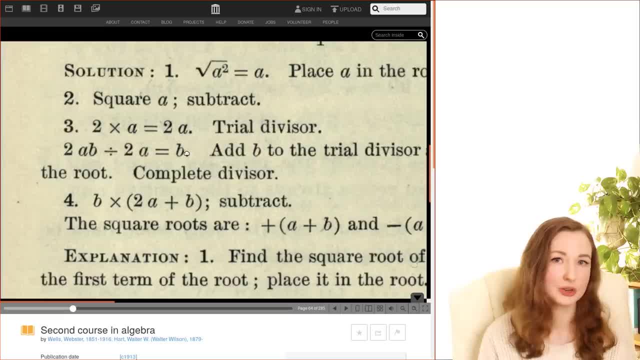 that juxtapositions should come before division when they set their rules. Well, one possibility is that they just didn't realize that it was contradictory, that what they were saying in that rule didn't agree with what they're actually doing in that book. Another possibility is that they did realize that it was a contradiction, but they 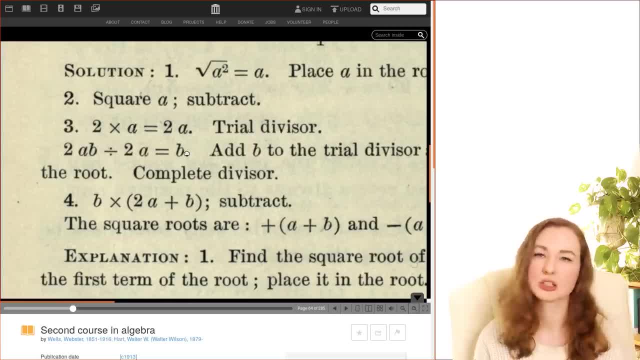 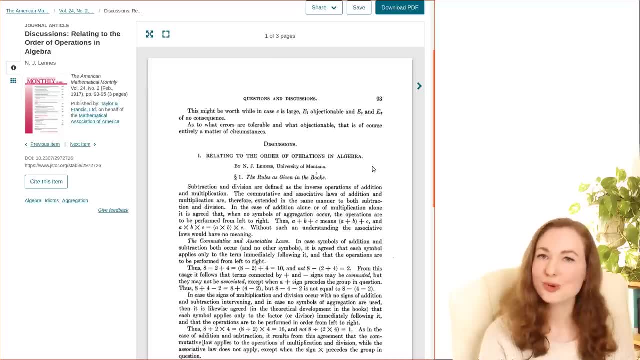 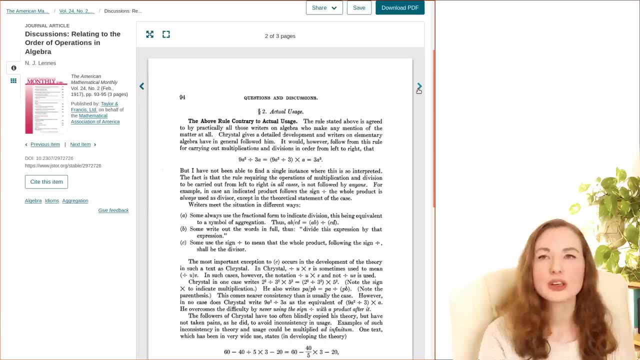 actually thought. you know, everyone already knows that juxtaposition comes before division. It's so well established that we don't even need to say it, But some authors of the time did notice the contradiction. There's this article by NJ Lennis, who was pointing out that the rule stated in these books is a 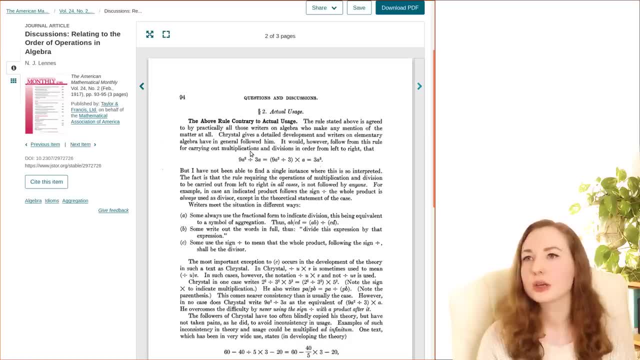 contradiction with the actual usage. So he was saying, like if we actually follow that rule, then you would find that, for example, 9a squared divided by 3a would equal 3a cubed, if you use the rule. that's written in the books but no one would interpret it in that manner. So the point I want to hammer: 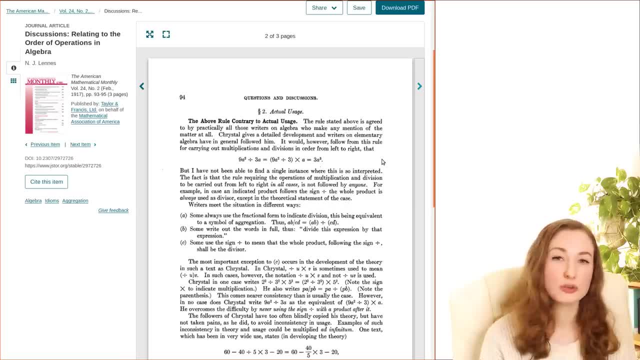 home here is that juxtaposition going before division was already well established well before anyone came up with this idea of PEMDAS. So at the time of writing of this, people were still arguing whether division or multiplication should be done first, But everyone agreed that 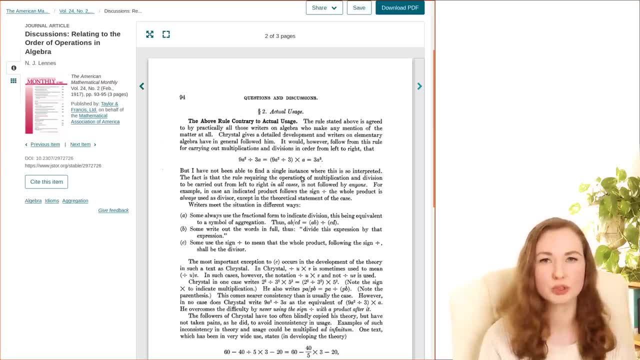 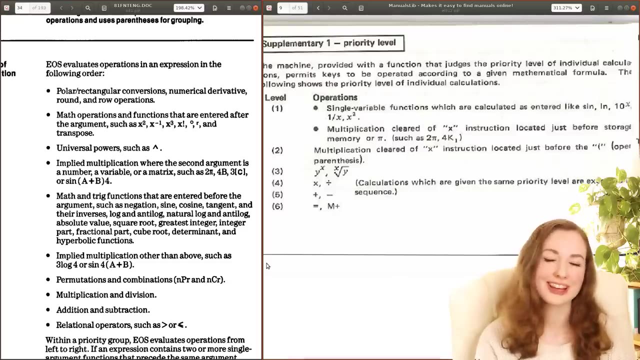 multiplication by juxtaposition always comes first, before division. Even the people who were saying that divisions and multiplication should be applied in the order that they occur from left to right In the early days of scientific calculators, they didn't actually support multiplication by juxtaposition at all. 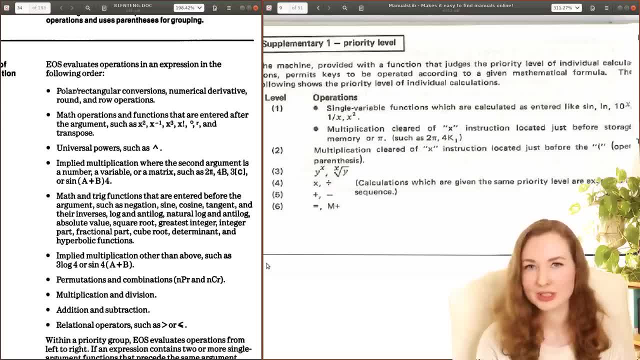 If you left out the time symbol, they just give you a syntax error. Now, the earliest one that I could find a manual for online that supports juxtaposition was the EL512, which was released in 1984.. This is from Sharp and they say they've got multiplication cleared of X instruction or times instruction. so 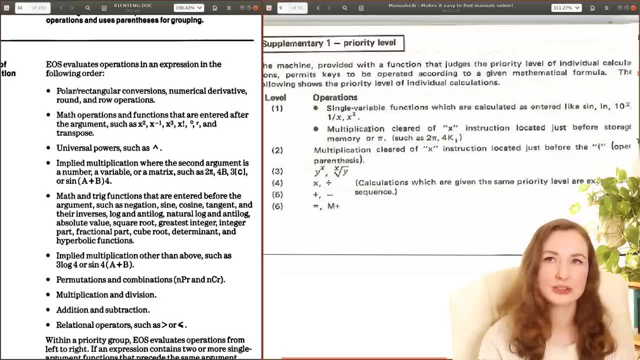 meaning multiplication where the times symbol has been left out. That's at a higher priority level than normal multiplication and division. And then here's the manual for the TI-81, which was released around 1990, and you can see they've put implied multiplication at a higher level. 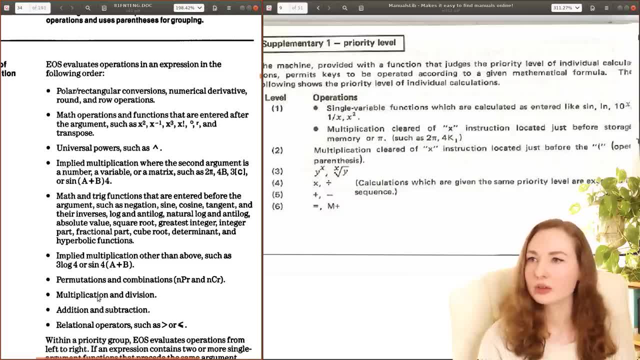 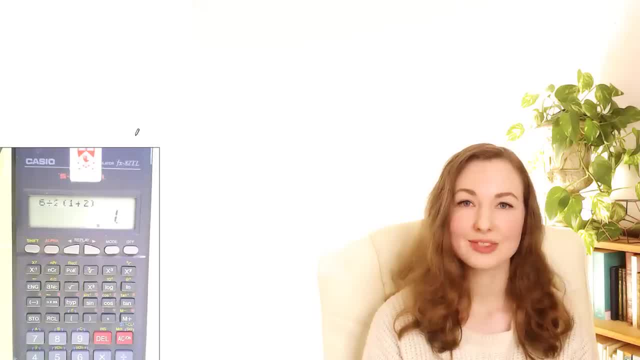 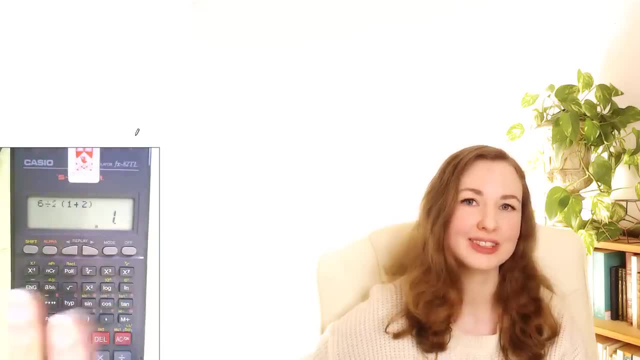 at that level and that level higher than regular multiplication and division. So both of these calculators are following Pejimdas. The early Casios followed Pejimdas as well. This is actually my old calculator that my parents bought for me around the year 2000, and you can see it's. 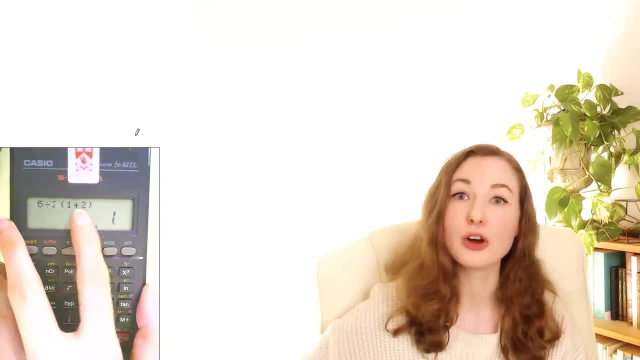 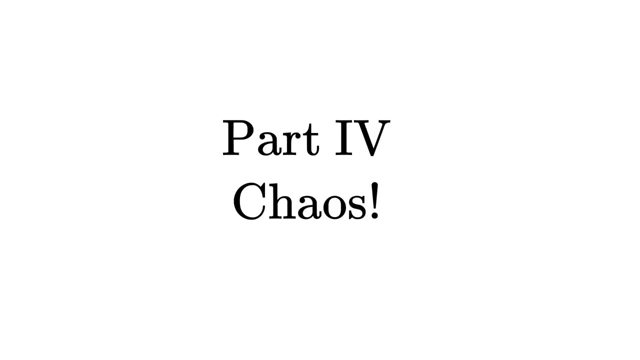 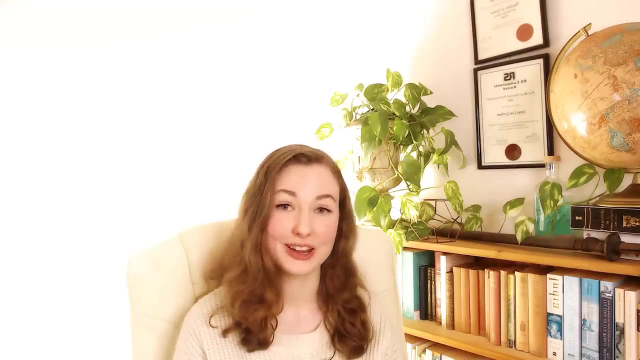 interpreting this as 2 times the 3, first making 6, and then 6 divided by that making 1.. So that's following Pejimdas as well. Then in the 90s and 2000s, everything changed. Texas Instruments came. 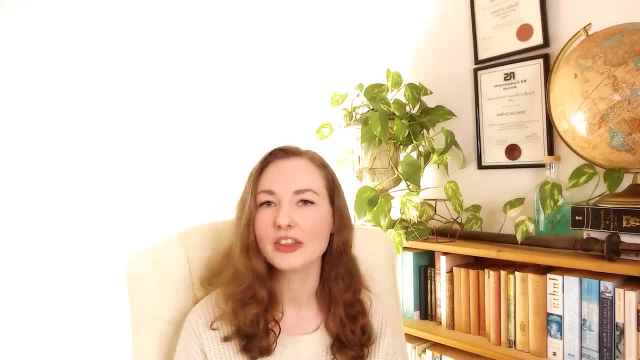 out with the TI-83 in 1996.. And that followed the PEMDAS rules, So they put the implied multiplication down all the way back to the same level as division. And then Casio came out with the FX-ES series in 2005, and that was. 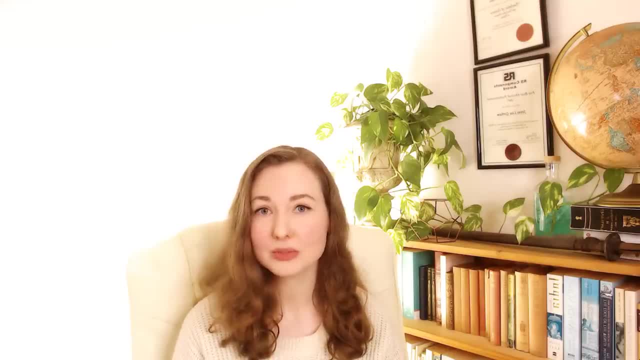 similarly PEMDAS. Sharp seems to have stuck with Pejimdas the whole way through, though Every calculator that I found from Sharp was Pejimdas, And then HP seems to be all over the place. Some follow PEMDAS, some of them follow Pejimdas, and I can't really see any sort of pattern to it. 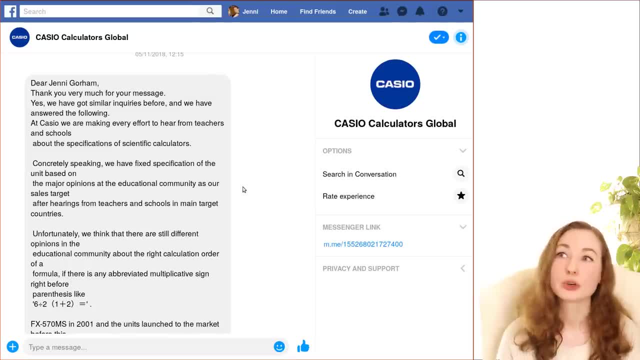 So why did this switch happen? Well, I've been corresponding with a representative from Casio who was saying that basically they make their calculators according to what teachers want. So they do various hearings with teachers in schools And they were saying that you know. 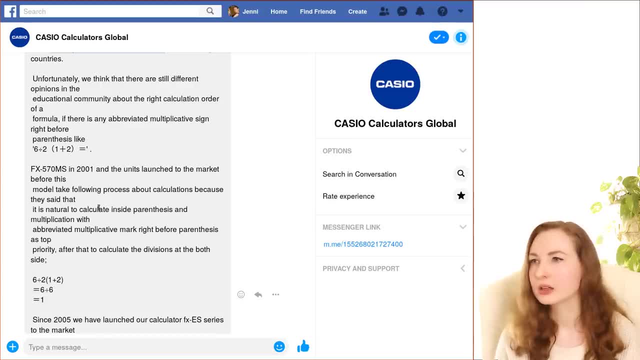 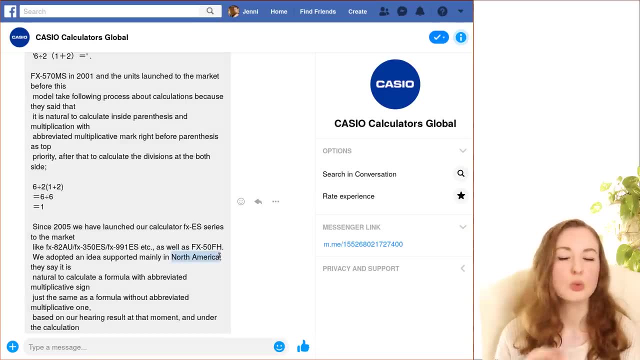 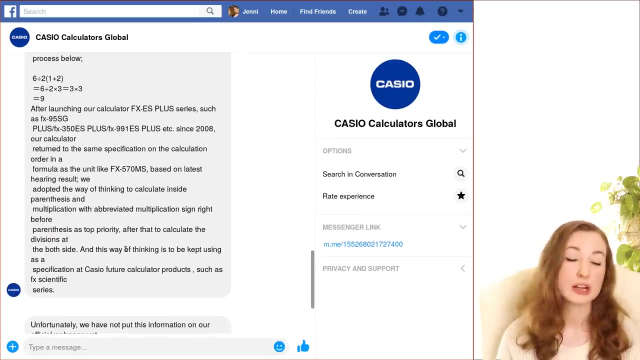 they started out with Pejimdas but then they switched to PEMDAS because teachers, and mostly teachers just from North America, wanted them to switch to PEMDAS. But now- actually after hearing from a wider range of people, they've switched back to Pejimdas. 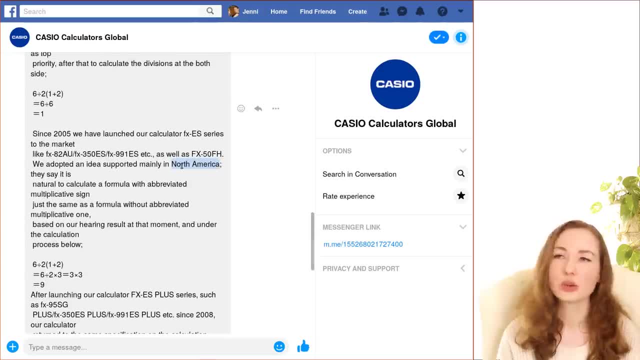 So I found it quite interesting that they said that it was just North American teachers who were pushing this idea of PEMDAS. I've been also talking to David Linkletter, who wrote an article about PEMDAS, about the same question of like what is six divided by two to the 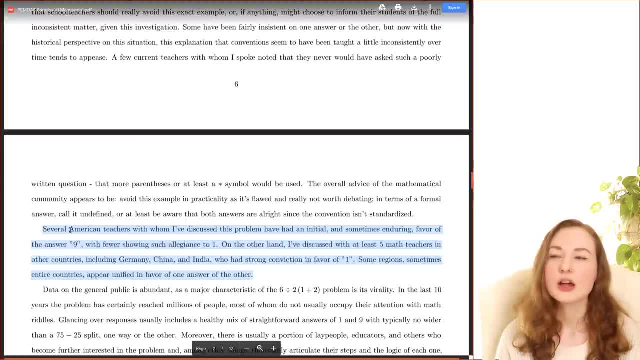 times one plus two, And he was saying something similar, that it was mostly the American teachers who were saying: okay, follow PEMDAS. the answer's nine, whereas teachers from the rest of the world, teachers that he's spoken to, from Germany, China and India, have said no, the answer is one. 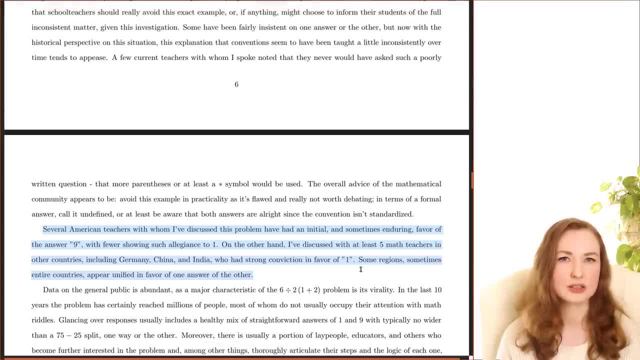 So I don't know why. that is why North American teachers are saying PEMDAS whereas the rest of the world is saying Pejimdas. And just to be clear, it's just the North American teachers who are in favor of PEMDAS, it's not mathematicians, or. 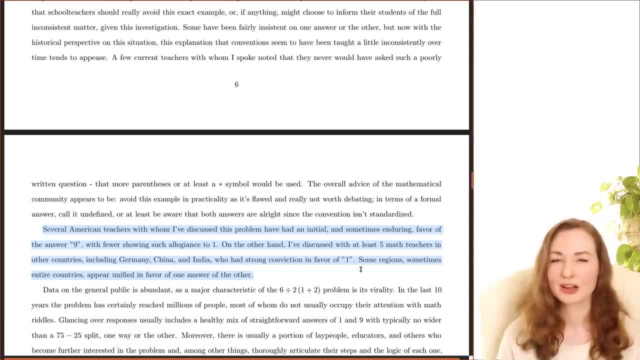 scientists or engineers from North America that are saying, okay, PEMDAS is the whole truth, it's a strict rule and you have to follow it, even with juxtaposition. There was also this statement from TI, which was: I just thought this was interesting because 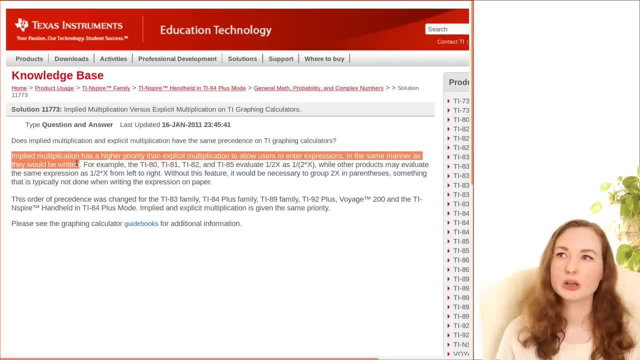 they were saying how they'd made the switch. but they were also saying that the actual convention when you're writing things down on paper is Pejimdas. So they were saying implied multiplication, like, should have a higher priority because that's how you would write things down, and but you know, 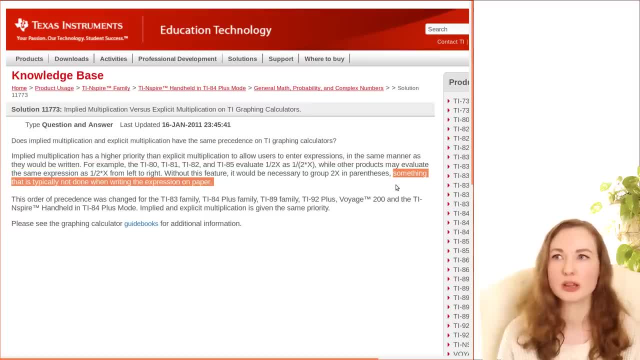 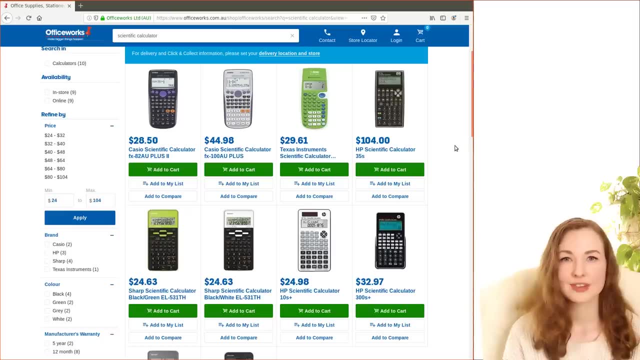 we've switched and now it's this different way that you wouldn't normally write on paper. Okay, enough about history. what about calculators that are still being made today? So I went by my local store to see what was available And whether they're following PEMDAS or Pejimdas these days. 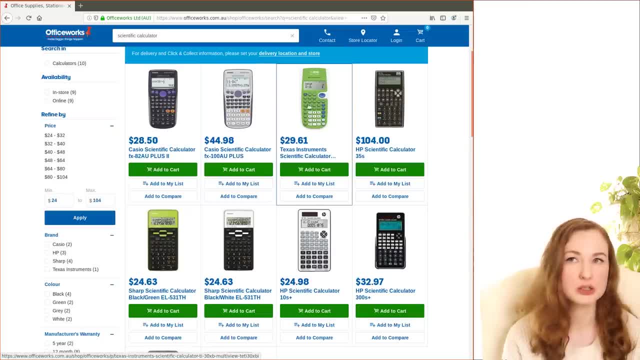 So the Casios are doing Pejimdas. the TI was the one that I showed at the start that one's doing PEMDAS. This one wasn't in stock and the manual, I think, doesn't actually mention in the priority levels implied multiplication. so I think that one might be PEMDAS, but I'm not sure. 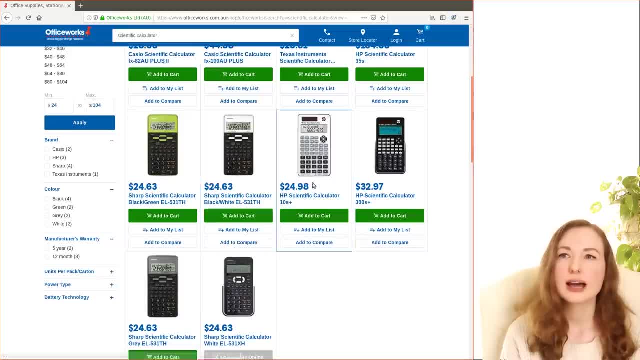 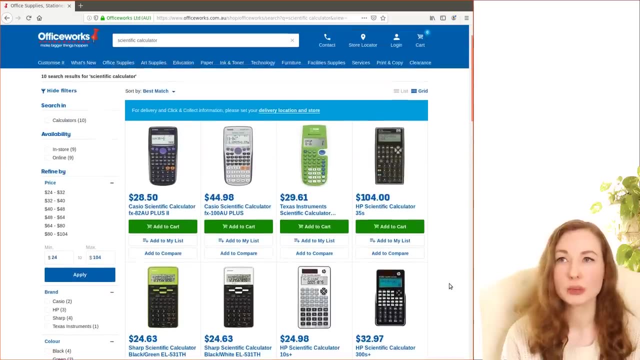 All of the sharps are Pejimdas. that one's Pejimdas, that one wasn't available, but from reading its manual I think that it's PEMDAS And these are all Pejimdas as well. those are sharps too, So most of them are following Pejimdas. 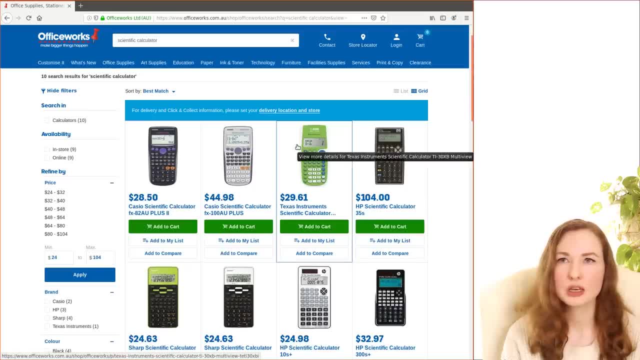 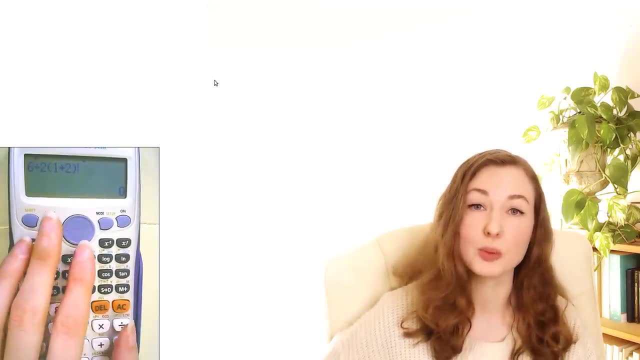 these days, with the exception of the TI and probably these HP ones that weren't even in stock so probably aren't sold as often as the others. Now I just want to show you what Casio is doing, because I think there's really a good solution to this problem. 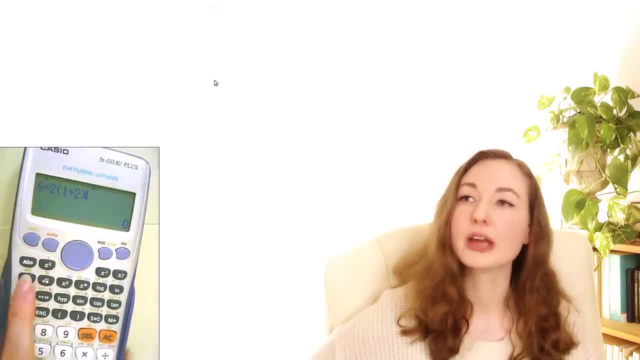 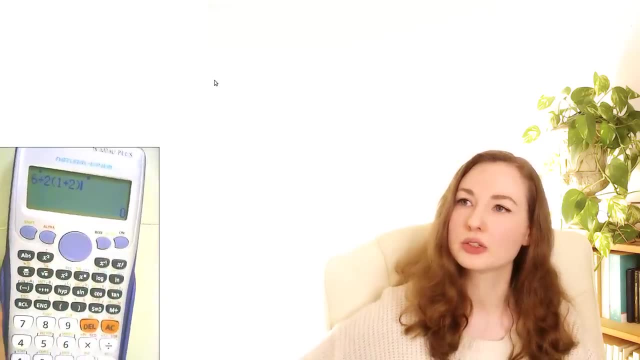 So this is a modern Casio FX100AU that I bought a few months ago. So if you type in 6 x 2 times 1 plus 2, let's see what happens. when I hit equals, It actually inserts brackets there. 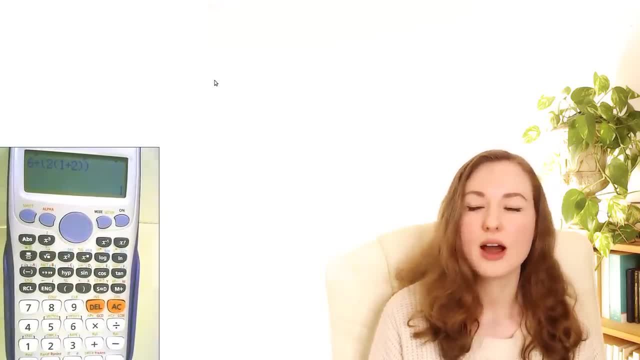 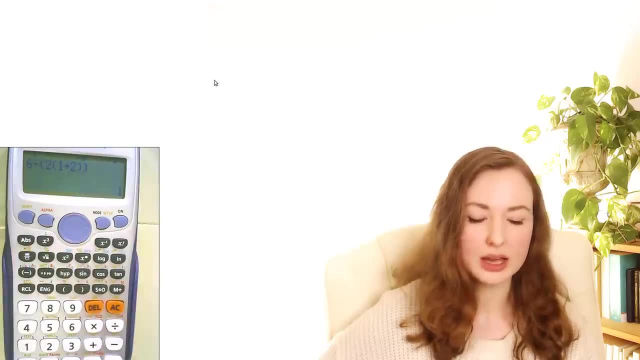 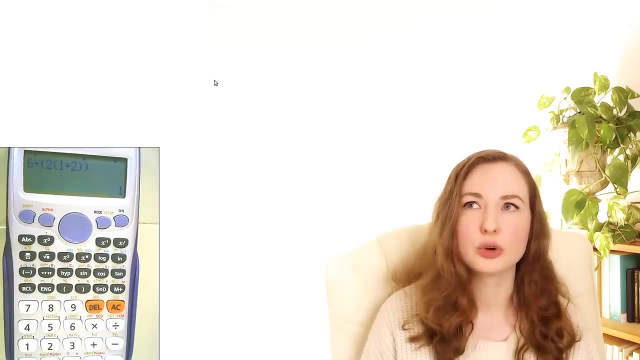 So, instead of just evaluating it some way and not letting you know, it actually tells you, by putting the brackets in, how it's interpreting that expression. So I think that is a really good solution, Unlike the HP and the TI and the sharps, which you know don't really explicitly tell you. 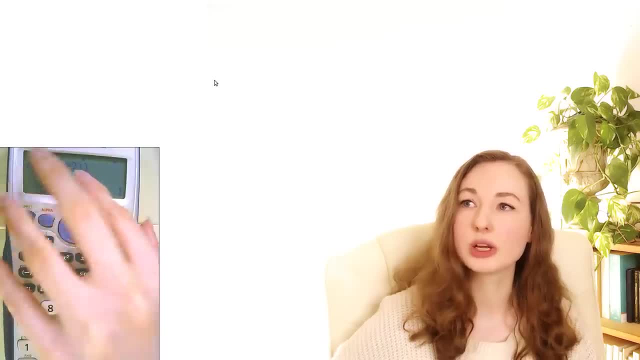 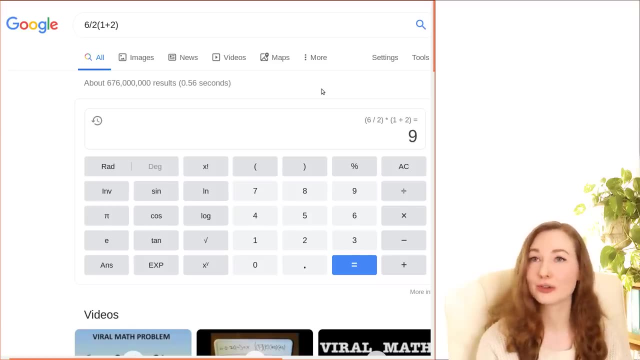 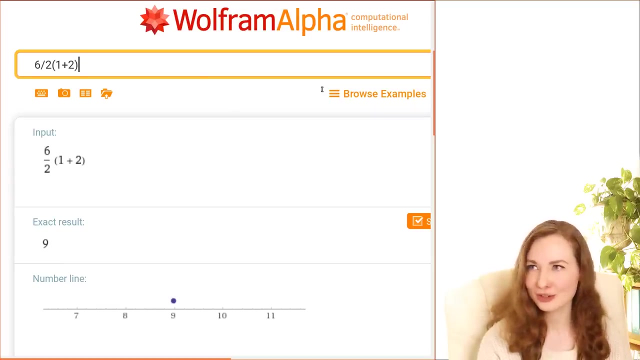 whether it's using PEMDAS or Pejimdas. the Casios will put in these brackets to let you know. As for online calculators, Google Calc follows PEMDAS, but WolframAlpha is really weird because, okay, here it's following PEMDAS, giving the answer of 9.. If you put it in a 6 divided, 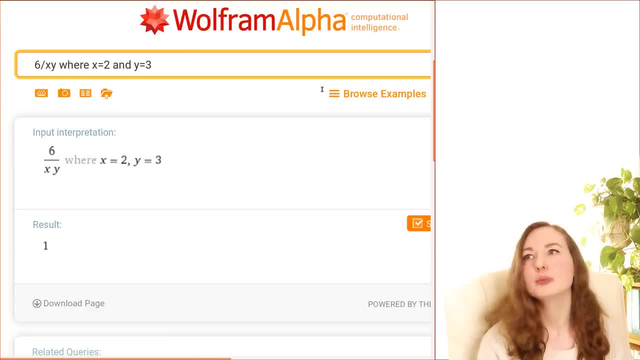 by 2 x. it's still following PEMDAS, but if you put in 6 divided by x- y, it will interpret that as, like Pejimdas, It interprets that as 6 divided by x and then divided by y as well, and gives the 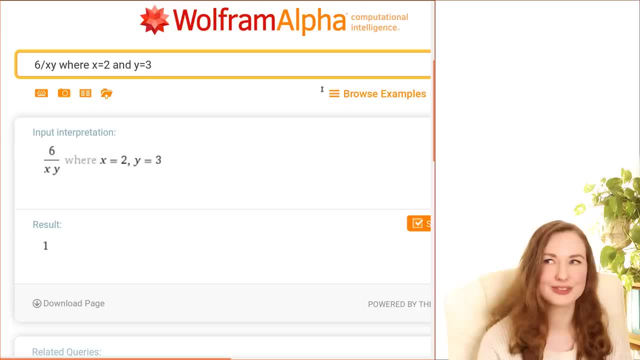 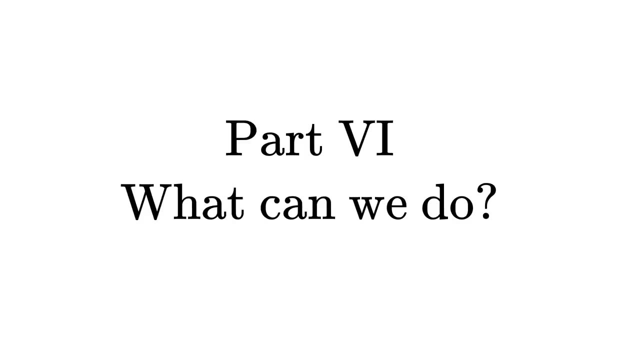 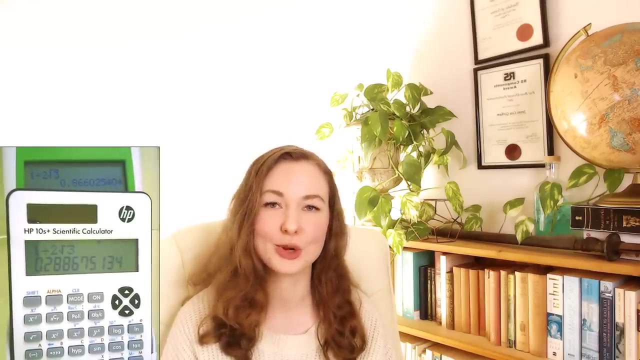 answer of 1.. So I'm not sure what kind of priority levels they're working with there, but they're a bit inconsistent, So I think we need to come to a conclusion. I think we need to come to a conclusion about which one of these is correct. 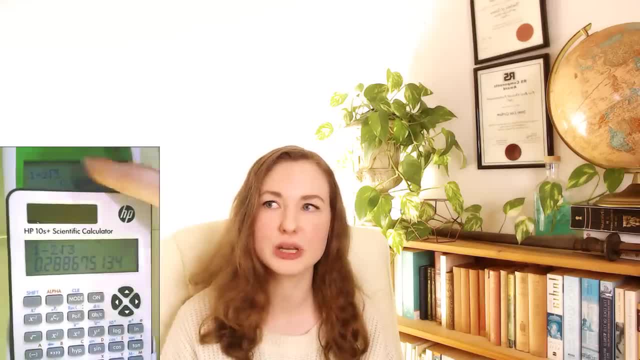 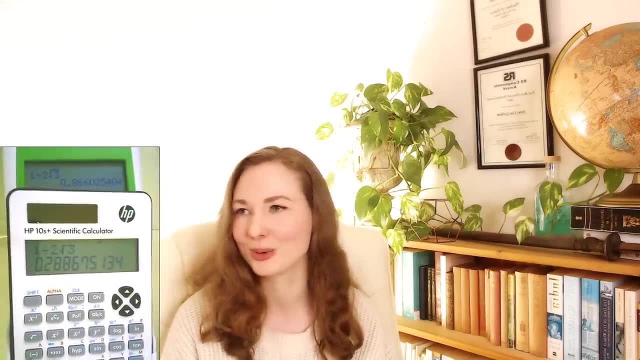 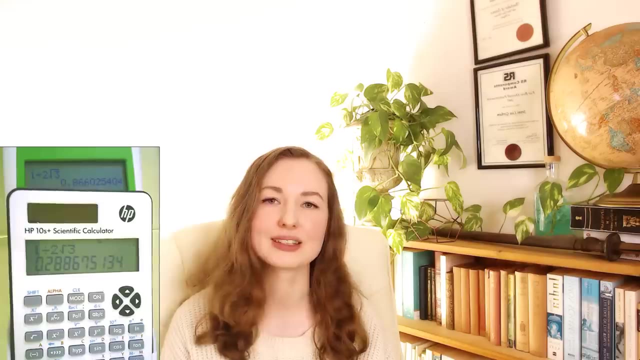 Do we interpret 1 divided by 2 root 3 as half of root 3, or do we interpret it the way that the majority of mathematicians, scientists and engineers would interpret it? So I'm firmly in favour of the Pejimdas Now. in my first video that I made on this, I was arguing based on usage. 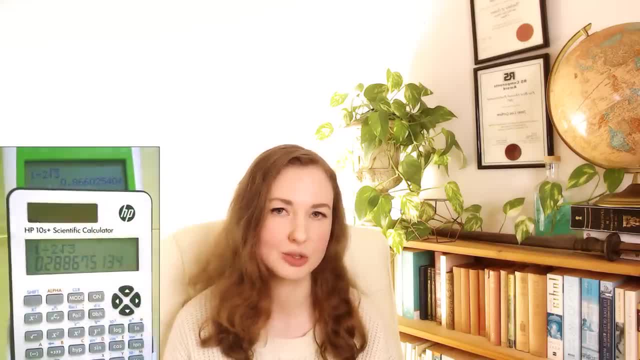 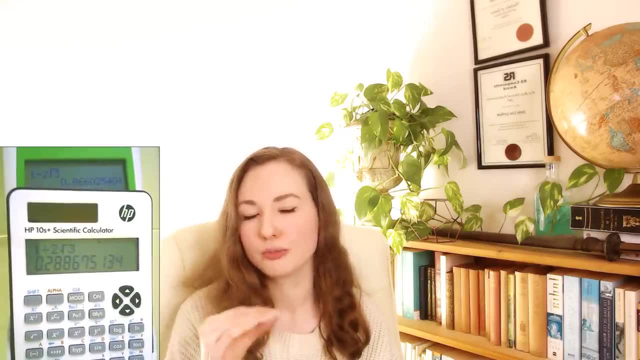 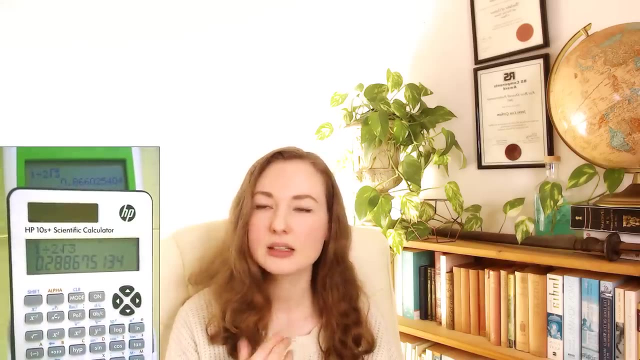 like. this is how mathematicians interpret it. this is therefore, this is the rule. Now, a lot of people correctly pointed out that if there is a strict rule of PEMDAS, then you know, mathematicians just shouldn't be lazy, they should use brackets or something. Now, I think that this comes from a 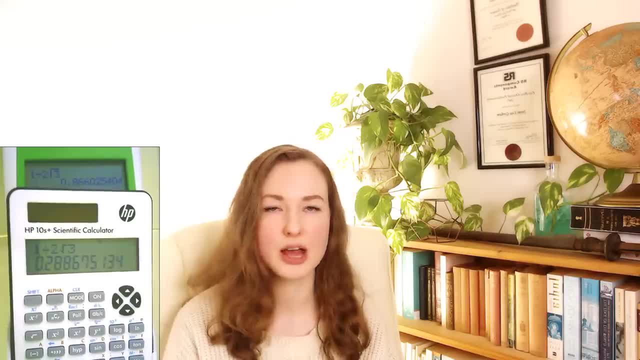 misconception that mathematicians have gotten together and decided: okay, PEMDAS is the rule. this is a strict rule. we should all follow this. That has not happened. PEMDAS was something that some educator wrote down as as as: 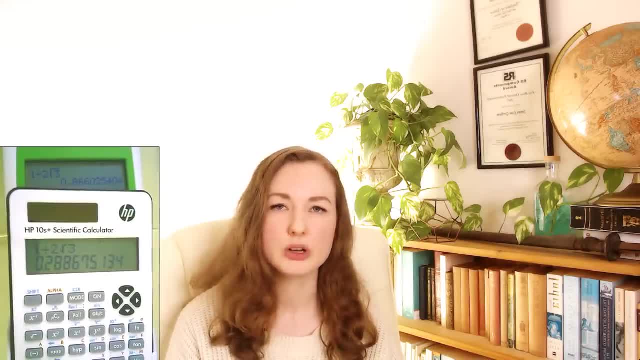 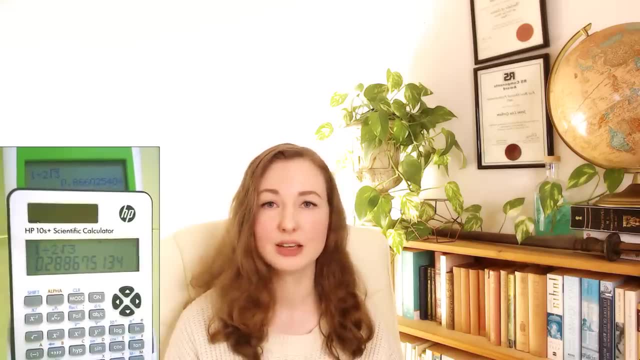 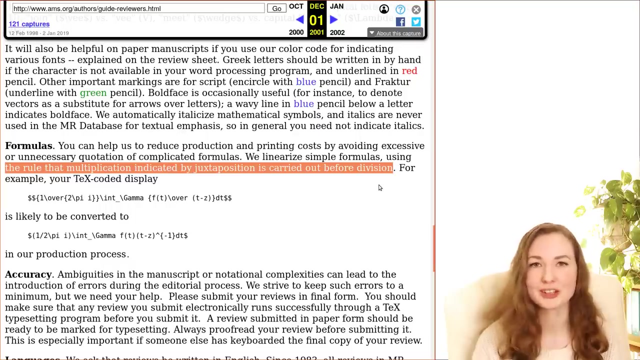 as either as an oversimplification or because they didn't understand the actual rules of mathematics. Mathematicians have not decided in any sort of way that multiplication and division should always have the same precedence, even if it's by juxtaposition. In fact, if you want to see some official statements from mathematicians or scientists, then we could. 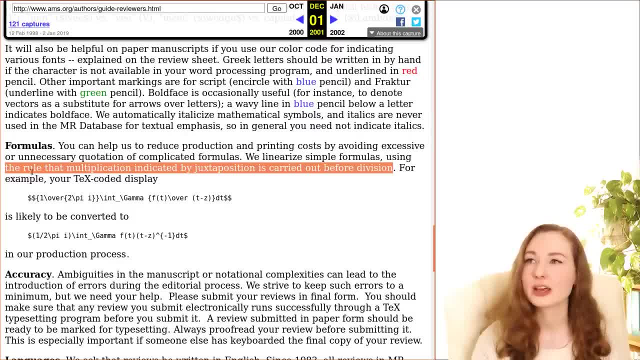 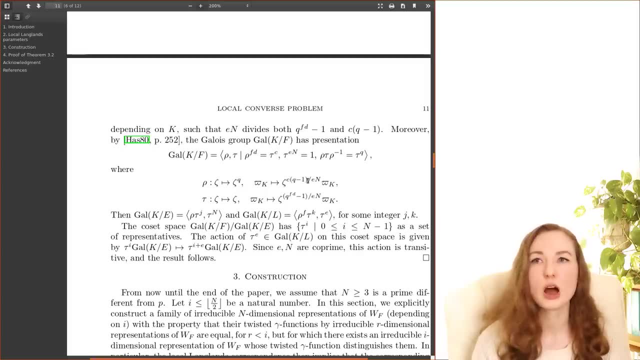 look at the American Mathematical Society style guide which said the rule that multiplication is indicated by juxtaposition is carried out before division. It actually doesn't say that anymore. this is a past style guide, but they do still use that rule. For example, here is a recent article.